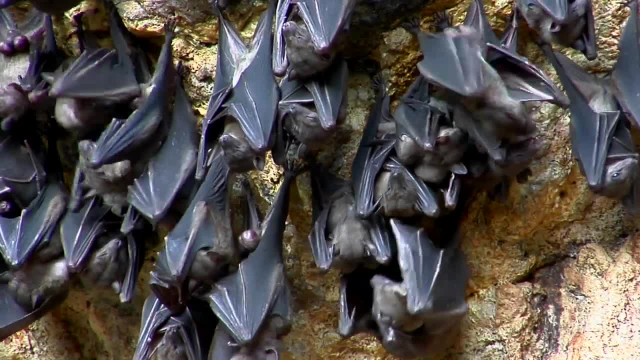 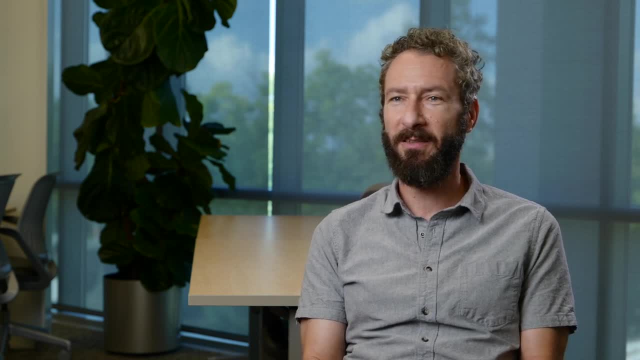 can help us trace the kind of origins of these viral outbreaks. Here there's this nice mix of you're getting lots of people who study informatics, so lots of different domain expertise. The biology department here is also very strong. There's a lot of people that have really interesting. 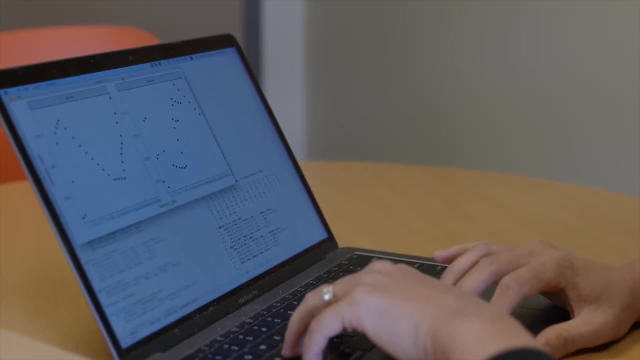 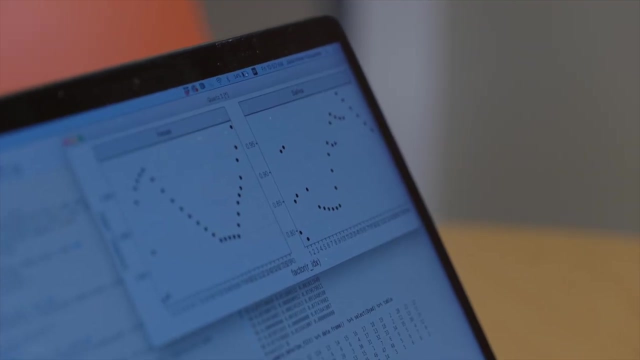 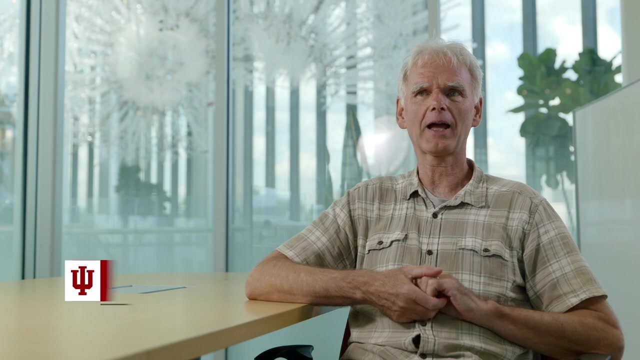 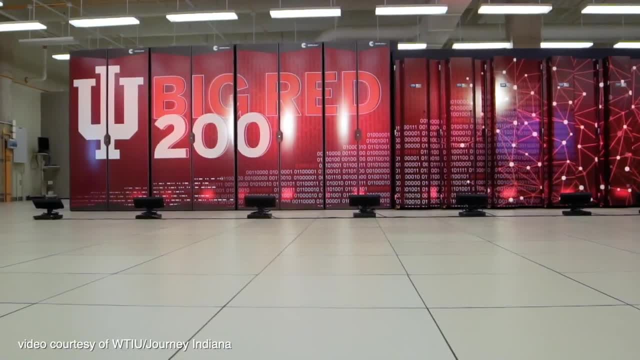 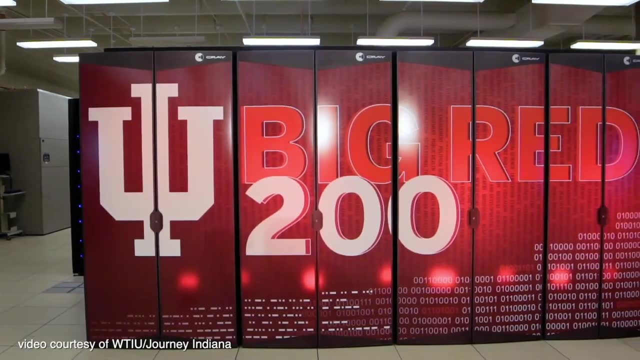 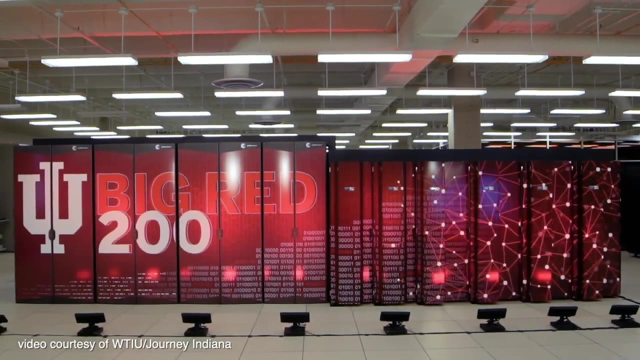 The computing resources at IU are really amazing. So we have free access to all of Big Red 200, all of the graphics processing units that are in Big Red 200, so specialized for machine learning uses. It's just an amazing place to be able to take whatever idea you have and apply it to whatever. 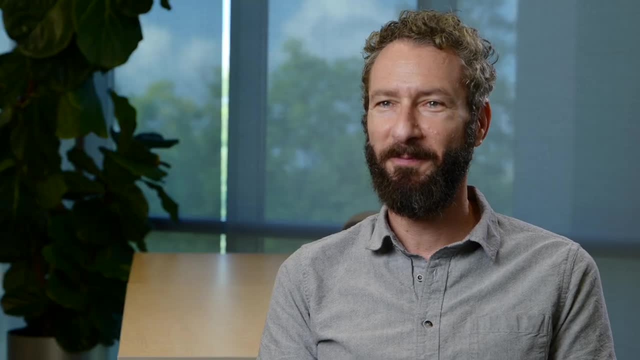 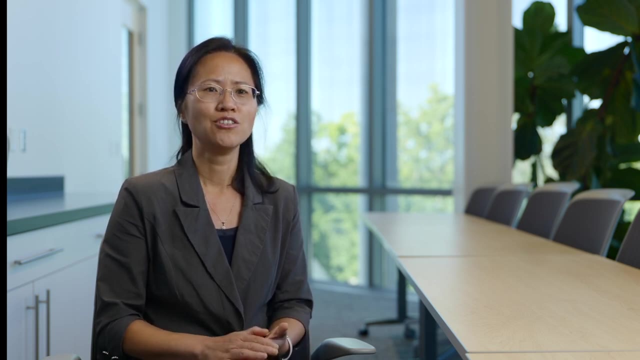 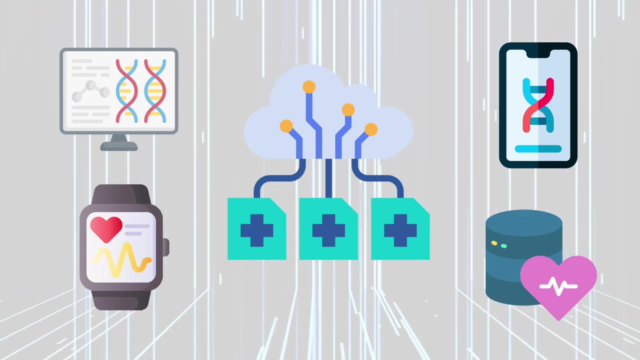 data you have and the computational resources are there. We have people working on cancer genomics. We have people working on microbiome research. like me, people working on genome privacy. I'm interested in privacy preserving technologies that allow us to analyze or mine massive. 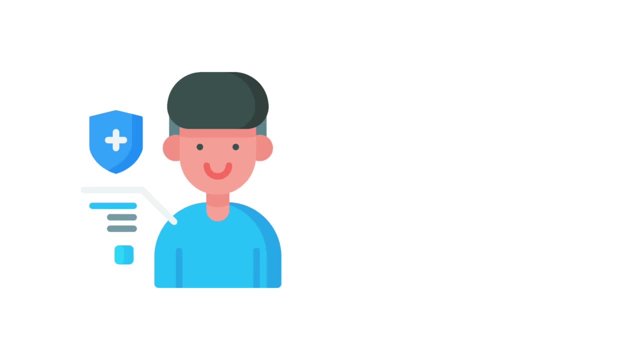 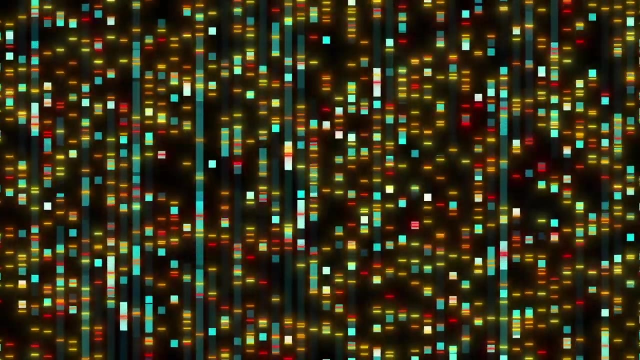 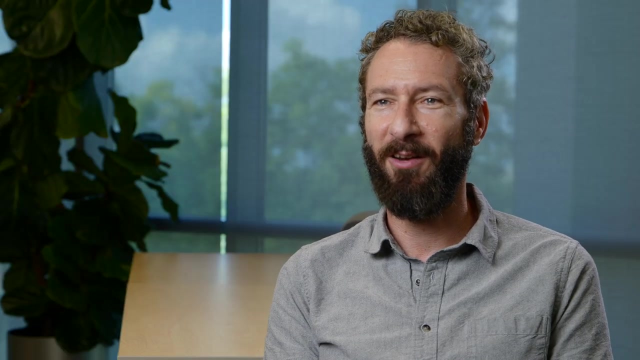 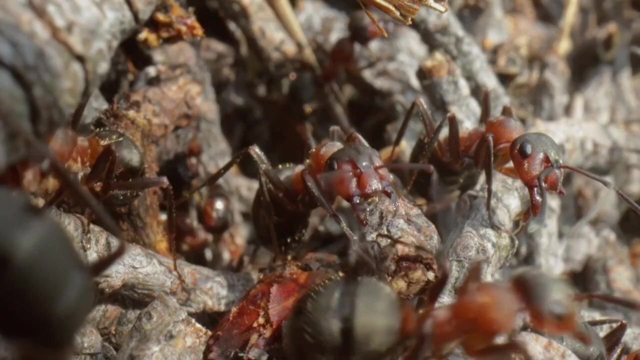 biomedical data without compromising the privacy of individual patients. I study the evolution of DNA sequences and genomes hold genomes. The changes that are making us all look different are occurring in the DNA. How do we harness this information to understand all of that? I'm looking at genome sequences, particularly in the plant genomes- social insects, bees. 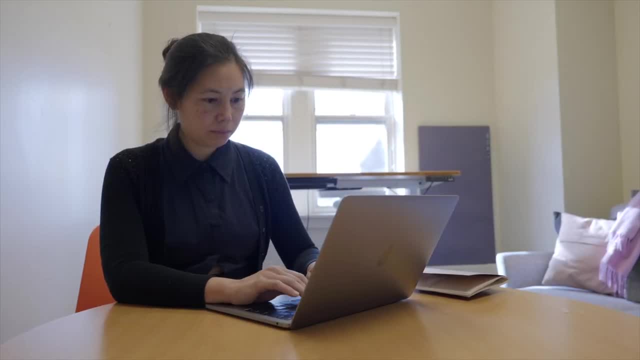 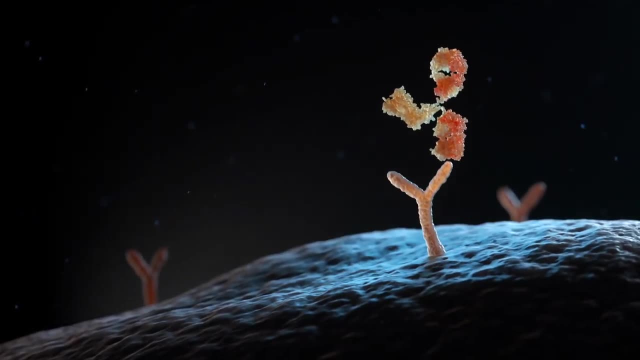 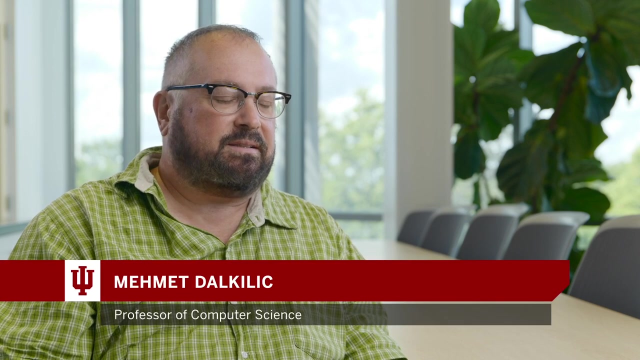 ants, that sort of thing. I've been working on a couple of immunology projects related to the development of B-cells, which are cells that make antibodies, which are the things that bind to and neutralize viruses. Currently, what I work on is called single-cell RNA sequencing. We look at the individual gene.